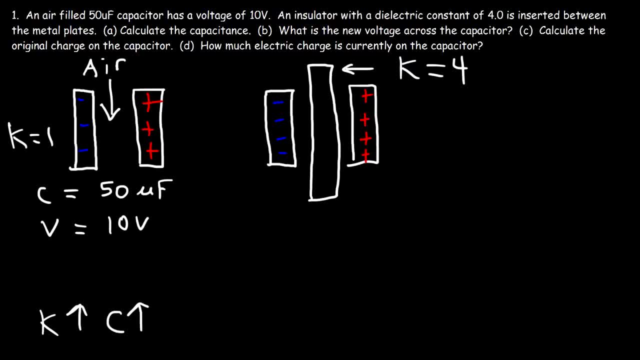 the K value. you need to know that the capacitance increases proportionally and the voltage decreases if the capacitor is not connected to a battery or some power source. If it's not connected to anything, the capacitance will go up, the voltage will go down and the charge simply stays the same. 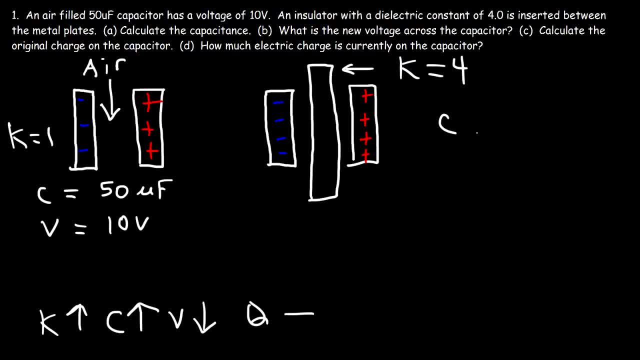 Now to calculate the new capacitance. let's call it CF or the final capacitance. it's equal to the original capacitance multiplied by the dielectric constant. So the original capacitance was 50 microfarads, and if we multiply it by 4,, 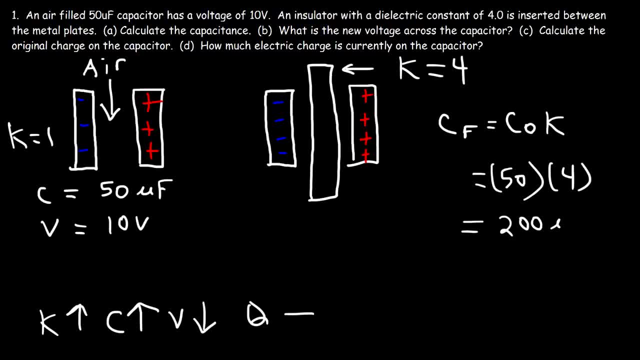 so the new capacitance is going to be 200 microfarads, So it increased by a factor of 4.. Now, what about the voltage? What is the new voltage? What is the new voltage across the capacitor? Well, to calculate the new, 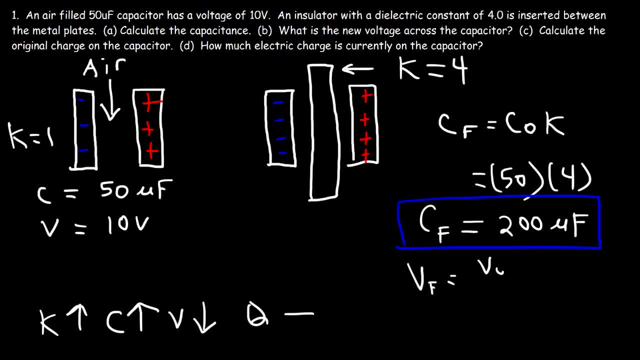 voltage. it's going to be the original voltage divided by K, because it's going to decrease. The original voltage was 10 volts and K is 4.. 10 divided by 4 is 2.5.. So that's the new voltage across the capacitor. Now let's move on to part C. 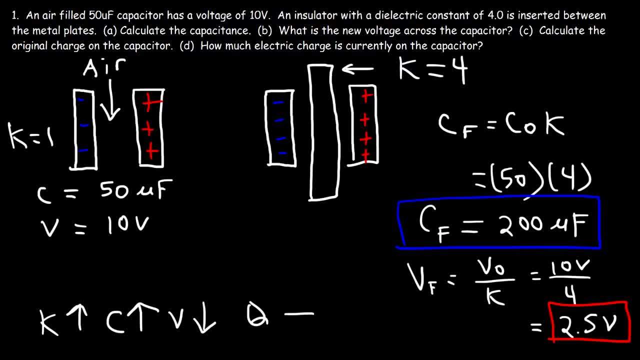 Calculate the original voltage. The original charge on the capacitor To calculate the electric charge is equal to CV, And so the original capacitance was 50 microfarads. and if we multiply that by 10 volts, 50 times 10, is 500. So if I keep the unit microfarads I'm going to 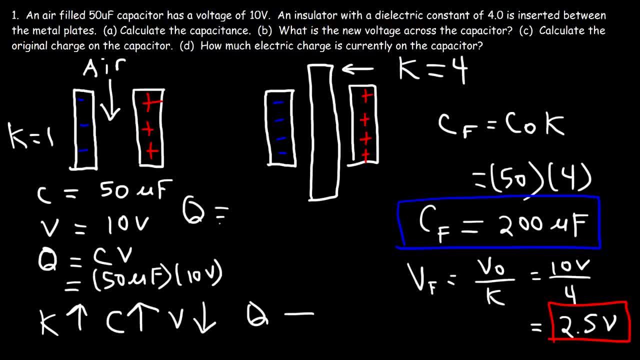 get microcoulombs. So the charge on this capacitor is 500 microcoulombs. That's the original charge. Now let's calculate the new charge using these new values. So let's see if I can fit it in somewhere. So Q equals CV. The new capacitance is 200 microfarads and 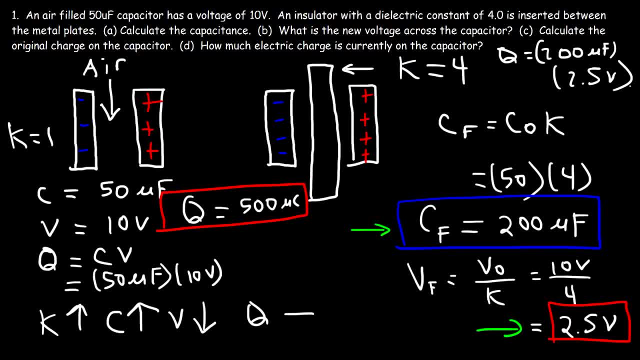 the new voltage is 2.5 volts. So if you take 200 and multiply by 2.5, you can get the same answer of 500 microcoulombs. So the charge doesn't change. Anytime you increase the dielectric constant, the capacitance will increase in value, the voltage will decrease. 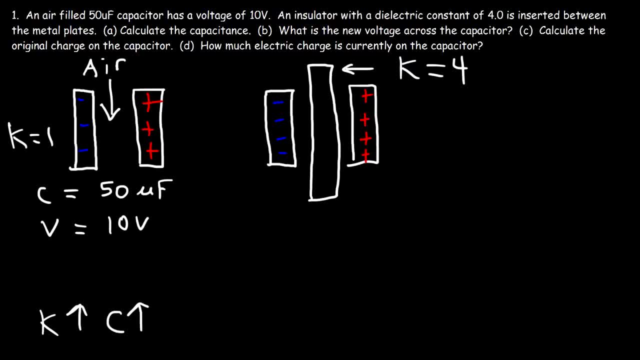 the K value. you need to know that the capacitance increases proportionally and the voltage decreases if the capacitor is not connected to a battery or some power source. If it's not connected to anything, the capacitance will go up, the voltage will go down and the charge simply stays the same. 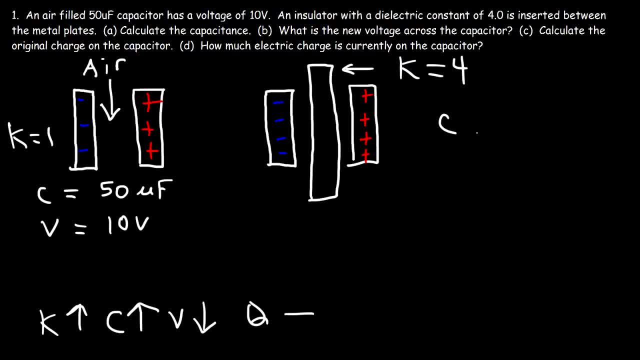 Now to calculate the new capacitance. let's call it CF or the final capacitance. it's equal to the original capacitance multiplied by the dielectric constant. So the original capacitance was 50 microfarads, and if we multiply it by 4,, 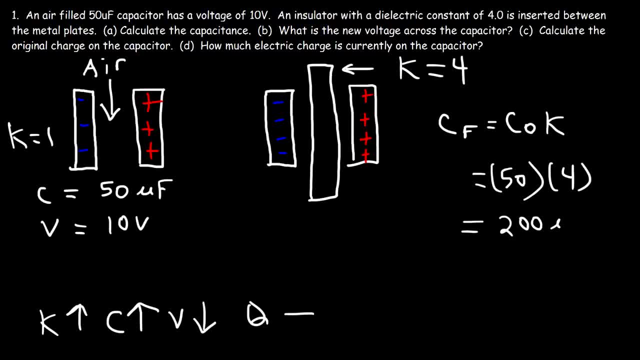 so the new capacitance is going to be 200 microfarads, So it increased by a factor of 4.. Now, what about the voltage? What is the new voltage? What is the new voltage across the capacitor? Well, to calculate the new, 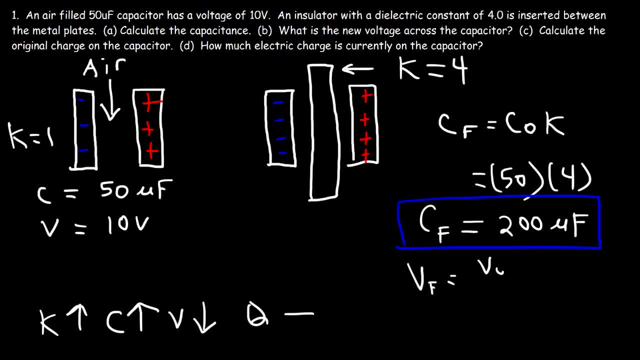 voltage. it's going to be the original voltage divided by K, because it's going to decrease. The original voltage was 10 volts and K is 4.. 10 divided by 4 is 2.5.. So that's the new voltage across the capacitor. Now let's move on to part C. 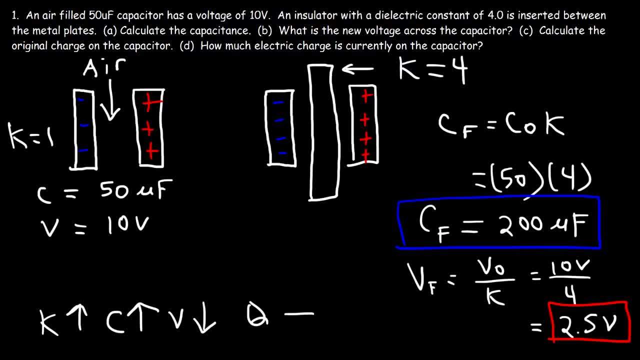 Calculate the original voltage. The original charge on the capacitor To calculate the electric charge is equal to CV, And so the original capacitance was 50 microfarads. and if we multiply that by 10 volts, 50 times 10, is 500. So if I keep the unit microfarads I'm going to 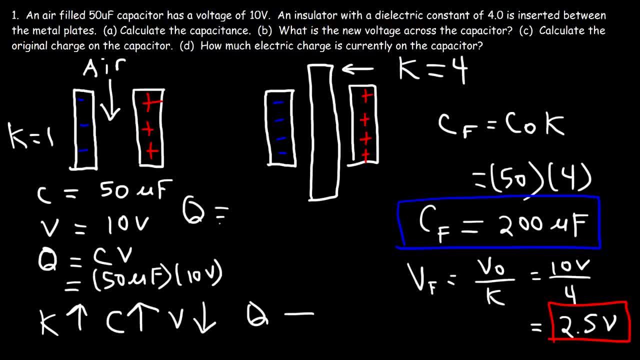 get microcoulombs. So the charge on this capacitor is 500 microcoulombs. That's the original charge. Now let's calculate the new charge using these new values. So let's see if I can fit it in somewhere. So Q equals CV. The new capacitance is 200 microfarads and 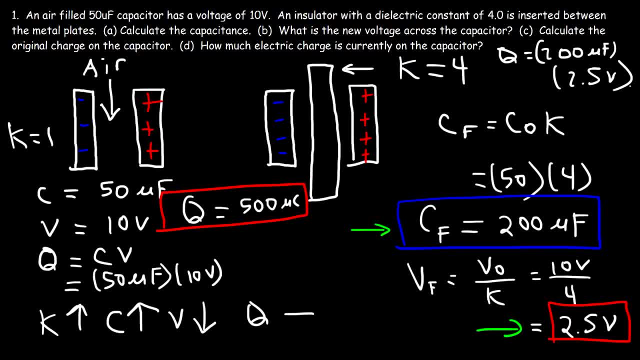 the new voltage is 2.5 volts. So if you take 200 and multiply by 2.5, you can get the same answer of 500 microcoulombs. So the charge doesn't change. Anytime you increase the dielectric constant, the capacitance will increase in value, the voltage will decrease. 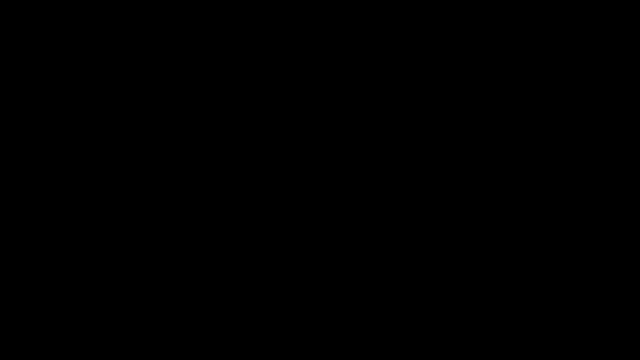 in value and the charge will stay the same. And it makes sense why the charge will stay the same. If we increase C and decrease V proportionally, these two will cancel, such that Q stays the same. Number two: a capacitor composed of two metal plates separated by an air gap of one millimeter. 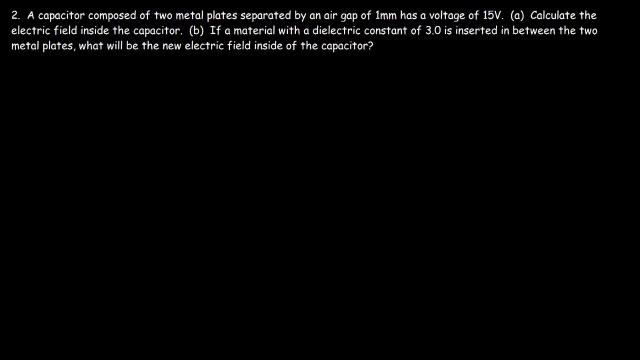 has a voltage of 15 volts. Calculate the electric field inside the capacitor. So let's say it's separated by a distance of one millimeter. This is going to be the positive plate and this is going to be the negatively charged plate, And so the capacitor has a voltage. 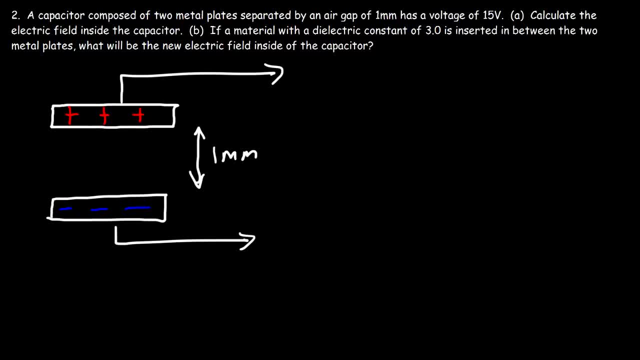 of 50.. Okay, Okay, All right, 15 volts. So calculate the electric field in between the two plates. To calculate the electric field is simply the voltage divided by the distance. So it's 15 volts divided by one millimeter, or .001 meters. 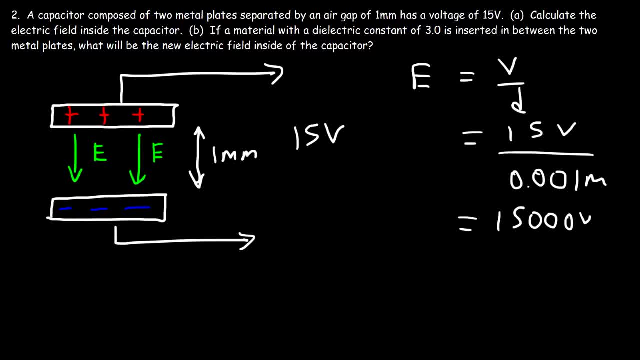 And so that works out to be 15,000 volts per meter. So that's the electric field inside the capacitor. Now let's move on to the next part. If a material with a dielectric constant of 3.0 is inserted in between the two metal plates, 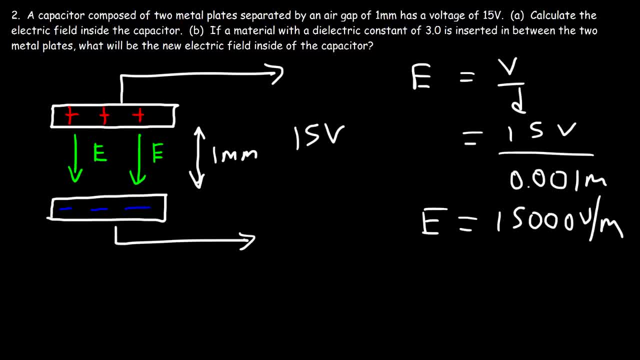 what will be the new electric field inside of the capacitor? So if we increase the dielectric constant of the capacitor, will the electric field increase or decrease? Well, we know that the voltage will decrease if it's not connected across the battery And the electric field is proportional. 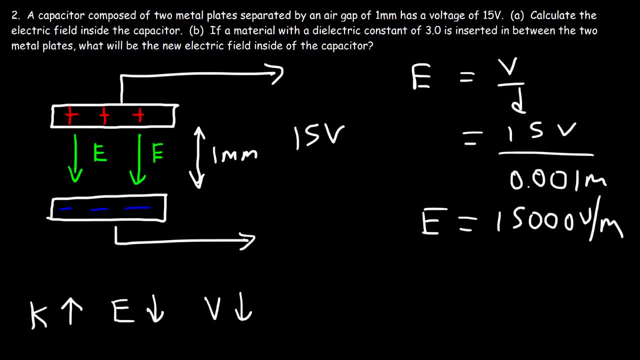 to the voltage, So therefore the electric field should decrease as well. So to calculate the new electric field, it's gonna be the original electric field divided by K, So that's gonna be 15,000 divided by three. And 15 divided by three is five. 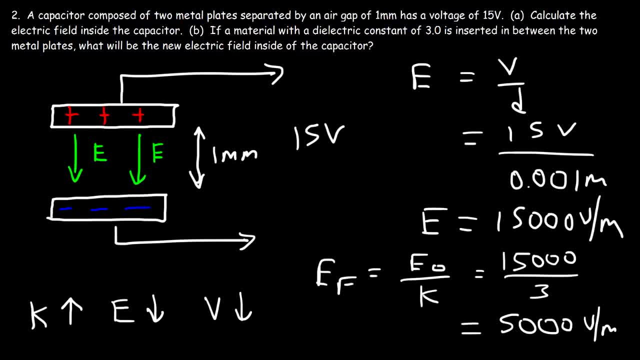 So it's now 5,000 volts per meter. Now what about the potential energy of the capacitor? If we increase the dielectric constant, what happens to the potential energy? The potential energy is one half QV. Now we know that if it's not connected across the battery, 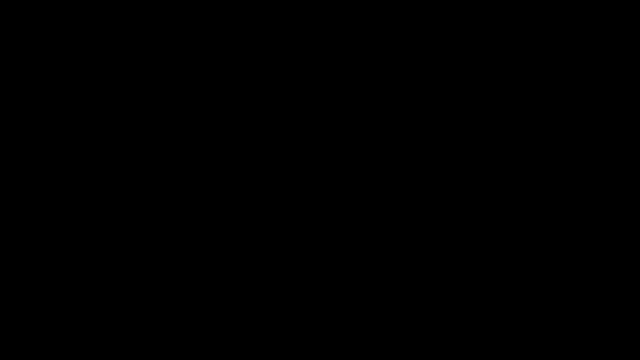 in value and the charge will stay the same. And it makes sense why the charge will stay the same. If we increase C and decrease V proportionally, these two will cancel, such that Q stays the same. Number two: a capacitor composed of two metal plates separated by an air gap of one millimeter. 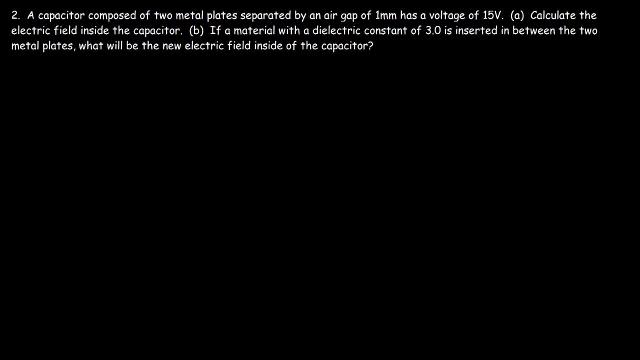 has a voltage of 15 volts. Calculate the electric field inside the capacitor. So let's say it's separated by a distance of one millimeter. This is going to be the positive plate and this is going to be the negatively charged plate, And so the capacitor. 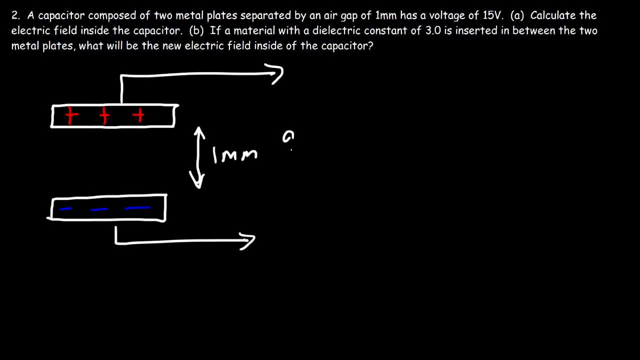 has a voltage of 15 volts. Okay, Okay, Okay, Okay. So we got a voltage of 15 volts, So calculate the electric field in between the two plates. To calculate the electric field, it's simply the voltage divided by the distance, So it's: 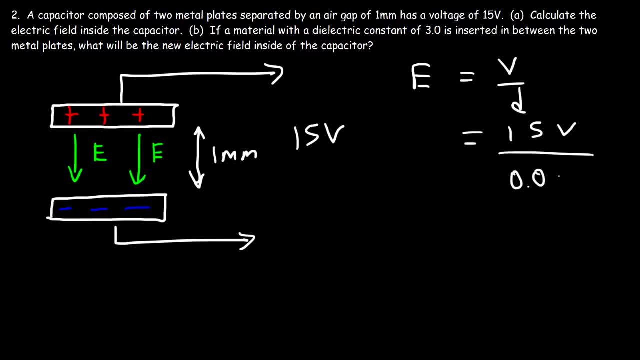 15 volts divided by 1 millimeter or 0.001 meters, And so that works out to be 15,000 volts per meter. So that's the electric field inside the capacitor. Now let's move on to the next part. If a material with a dielectric constant of 3.0 is inserted in between the two metal plates, what will be the new electric field inside of the capacitor? 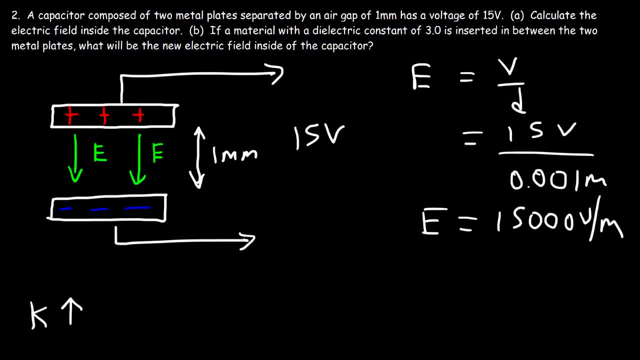 So if we increase the dielectric constant of the capacitor, will the electric field increase or decrease? Well, we know that the voltage will decrease if it's not connected across the battery and the electric field is proportional to the voltage. so therefore, the electric field should decrease as well. 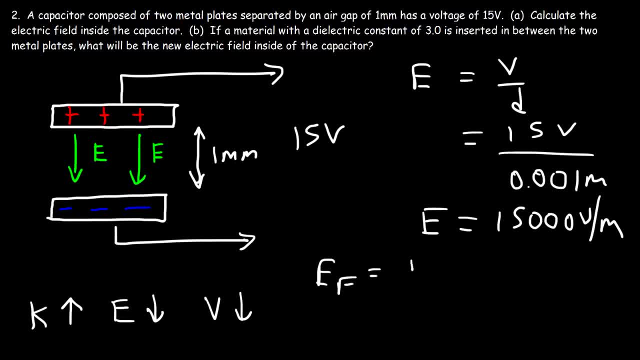 So to calculate the new electric field, it's going to be the original electric field divided by k, So that's going to be 15,000 divided by 3, and 15 divided by 3 is 5,, so it's now 5,000 volts per meter. 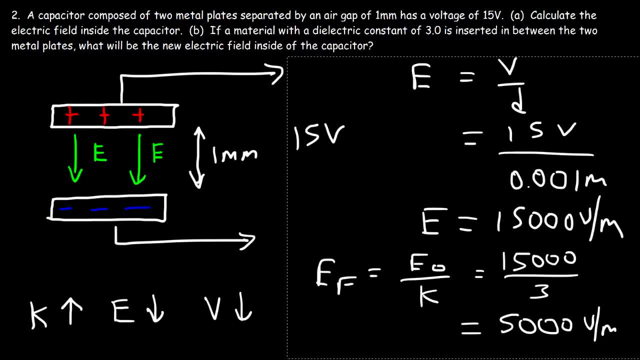 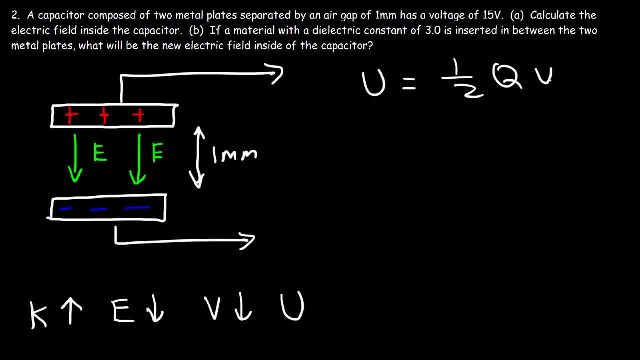 Now, what about the battery? What about the potential energy of the capacitor? If we increase the dielectric constant, what happens to the potential energy? The potential energy is 1 half qv. Now we know that if it's not connected across the battery, q stays the same. it doesn't change. 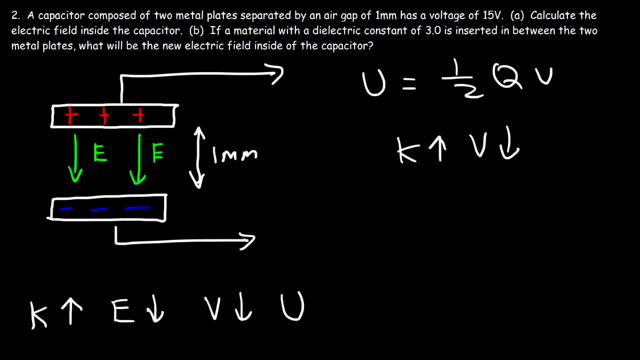 However, by adding a dielectric constant, the voltage decreases and so therefore the potential energy of the capacitor decreases. Now, once you insert an insulated material inside a capacitor, if that material has, let's say, polar molecules, initially these molecules won't be aligned. 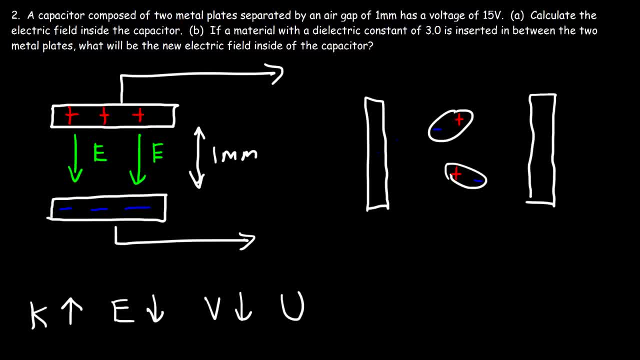 So they might look like this: Now, once you put them inside an electric field, these molecules won't be aligned. Now, once you put them inside an electric field, these molecules won't be aligned, will align themselves. The positive part of the molecules will be facing the negatively charged plate and the 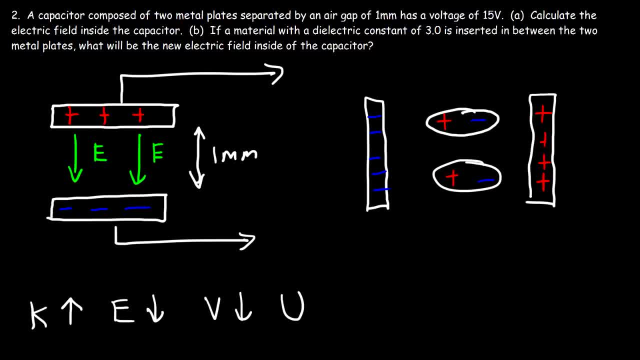 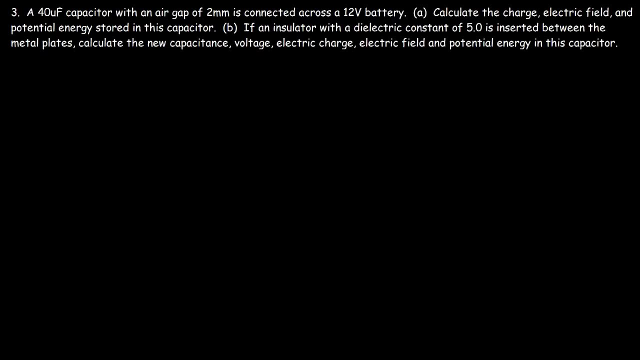 negative part of the molecules will be facing the positively charged plate, And so it takes energy for these molecules to realign themselves, And so that's one reason why the potential energy of the capacitor decreases. Now, in the last two problems we saw that if we add an insulator and if we increase, 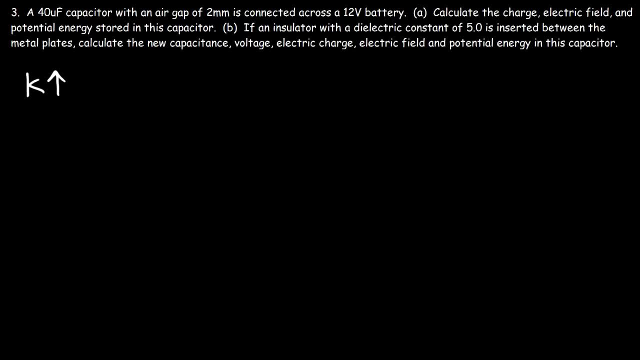 the dielectric constant of a capacitor that is not connected to a battery. the capacitance increased proportionally, the voltage decreased, the electric charge remained the same, the electric field decreased and the potential energy stored in a capacitor decreased. Now let's see what's going to happen if we add an insulator material. 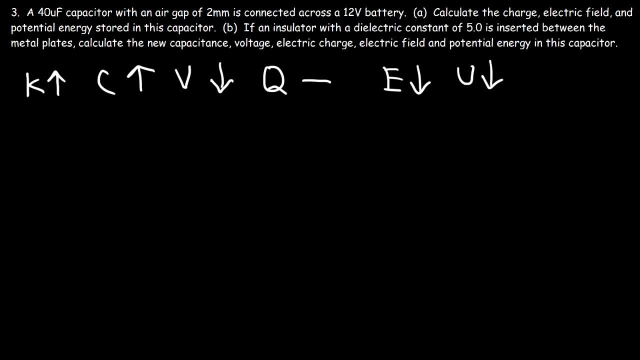 Now let's see what's going to happen if we add an insulator material to a capacitor that is connected to a battery, And let's say that the battery remains connected to the capacitor- It's not going to be disconnected at any point. So let's go ahead and try this. 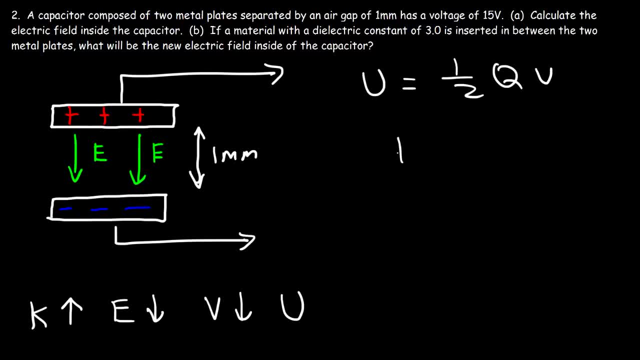 Q stays the same, it doesn't change. However, by adding a dielectric constant, the voltage decreases And so, therefore, the potential energy of the capacitor decreases. Now, once you insert an insulated material inside a capacitor, if that material has, let's say, polar molecules, 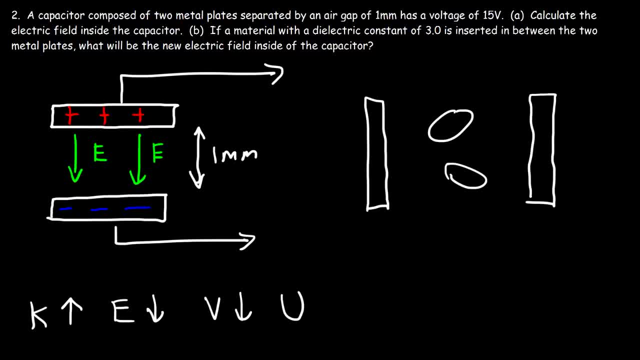 initially, these molecules won't be aligned, So they might look like this: Now, once you put them inside an electric field, these molecules will align themselves. The positive part of the molecules will be facing the negatively charged plate And the negative part of the molecules will be facing the positively charged plate. 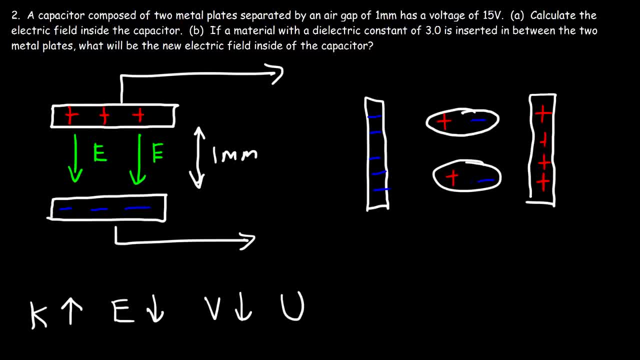 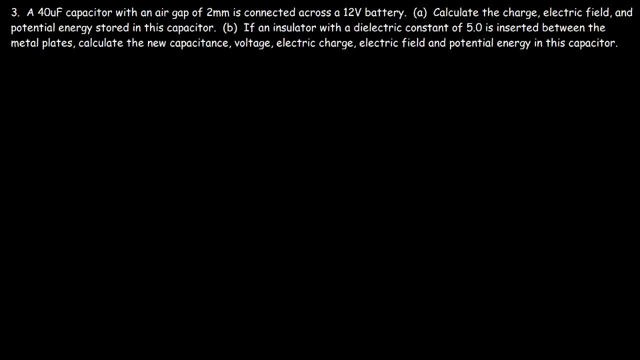 And so it takes energy for these molecules to realign themselves, And so that's one reason why the potential energy of the capacitor decreases. Now, in the last two problems we saw that if we add an insulator and if we increase the dielectric constant of a capacitor, 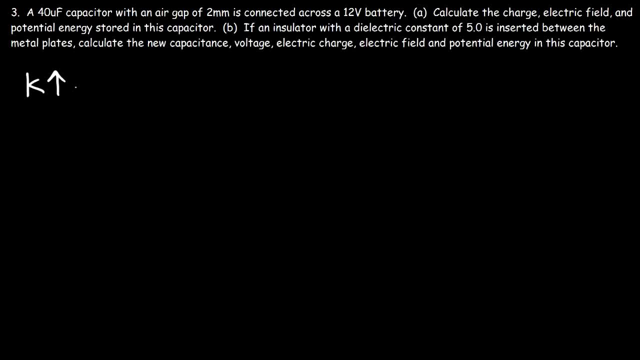 that is not connected to a battery. the capacitance increased proportionally, the voltage decreased, the electric charge remained the same, the electric field decreased and the potential energy stored in a capacitor decreased. Now let's see what's going to happen if we add an insulated material. 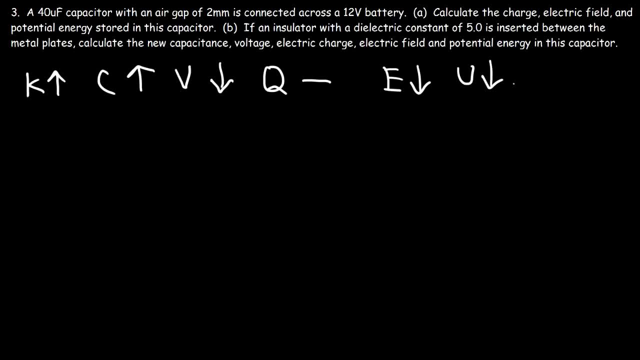 to a capacitor that is connected to a battery. Now let's say that the battery remains connected to the battery, to the capacitor. it's not going to be disconnected at any point. so let's go ahead and try this. so part a calculate the charge, electric field and potential. 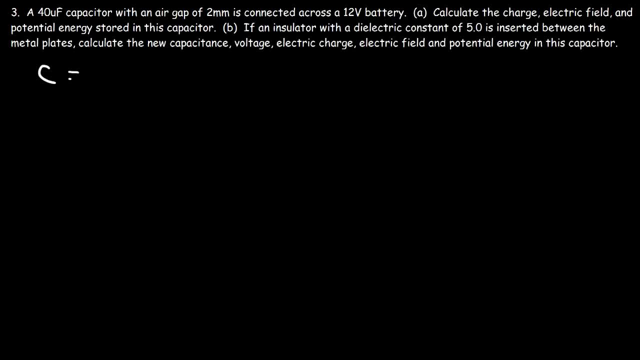 energy stored in this capacitor. so right now the capacitance is 40 micro farads. the voltage is 12 volts. so to calculate the charge, it's C times V, so it's 40 micro farads multiplied by 12 volts. so 4 times 12 is 48, so 40 times 12 must be. 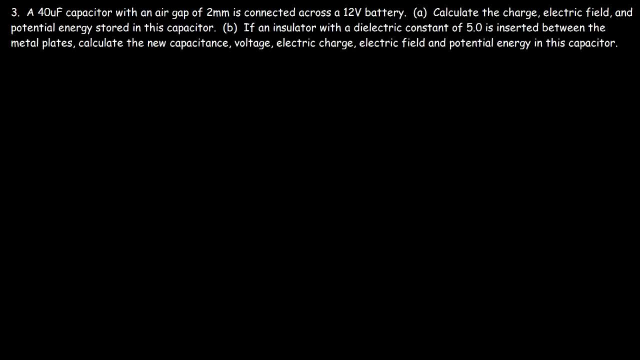 So part A, calculate the charge, electric field and potential energy stored in this capacitor. So right now the capacitance is 40 microfarads, The voltage is 12 volts, So to calculate the charge It's C times V, So it's 40 microfarads multiplied by 12 volts. 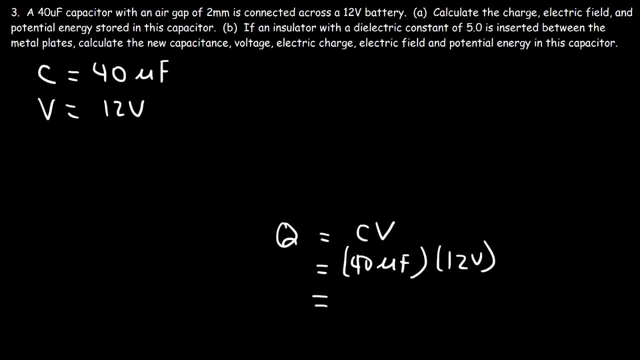 So 4 times 12 is 48. So 40 times 12 must be 480. So the electric charge is going to be 480 microcoulombs. The electric field is going to be the voltage divided by the separation distance, so we: 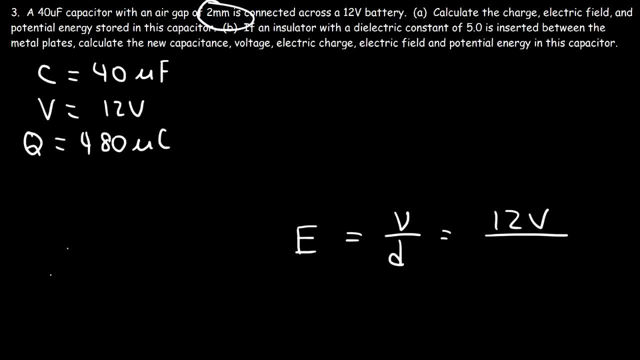 have a voltage of 12 and the separation distance is 2 millimeters or .002 meters, And so the electric field is 6,000 volts per meter. The potential energy is going to be 1 half QV. You could also calculate it using this 1 half Cv squared. 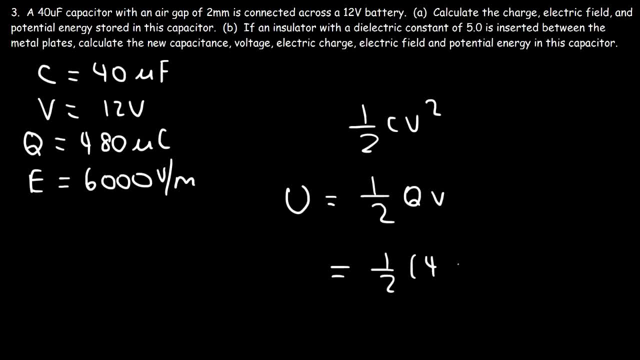 So you can use that formula too. The charge is 480 microcoulombs multiplied by a voltage of 12 volts. So because this is going to be in a micro, this answer is in millijoules. I mean microjoules. 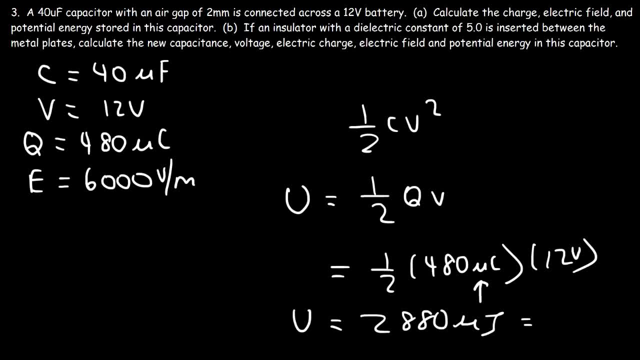 So this is 2880 microjoules, Which, if you multiply that by 1,000, that's 2.88 millijoules. So that's 480 microcoulombs multiplied by a voltage of 12 volts. 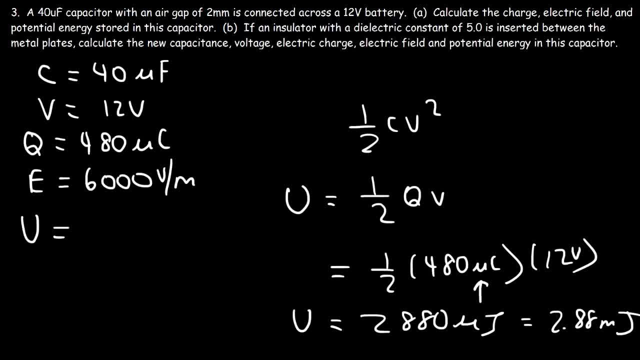 So you can use that formula too. The charge is 480 microcoulombs multiplied by a voltage of 12 volts. So that's the potential energy stored in this capacitor. Now let's move on to part B. So if we add an insulator with a dielectric constant of 5, what's going to be the new? 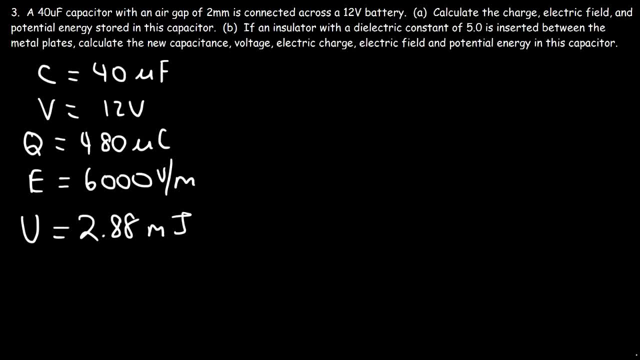 capacitance, voltage, electric charge, electric field and potential energy in this capacitor. Well, we know that. We know that the capacitance will increase. The new capacitance is going to be the original one times K, So it's going to be 40 microfarads over 5.. 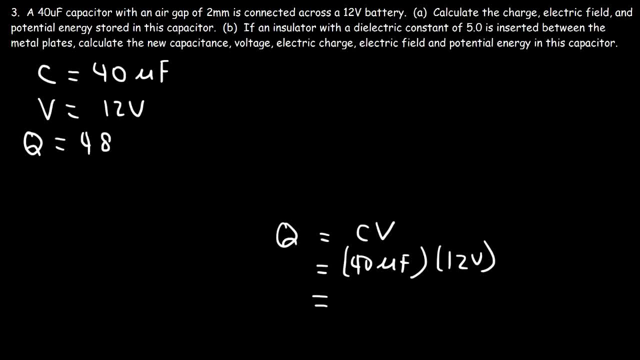 480, so the electric charge is going to be 480 micro coulombs. the electric field is going to be the voltage divided by the separation distance, so we have a voltage of 12 and the separation distance is 2 millimeters or 0.002 meters, and so the electric field is 6000 volts per 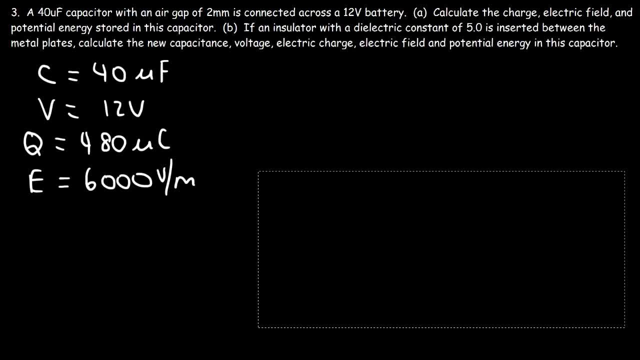 meter. the potential energy is going to be 1 half QV. you could also calculate it using this 1 half CV squared, so you can use that formula too. the charge is 480 micro coulombs multiplied by a voltage of 12 volts. so because this is going to, 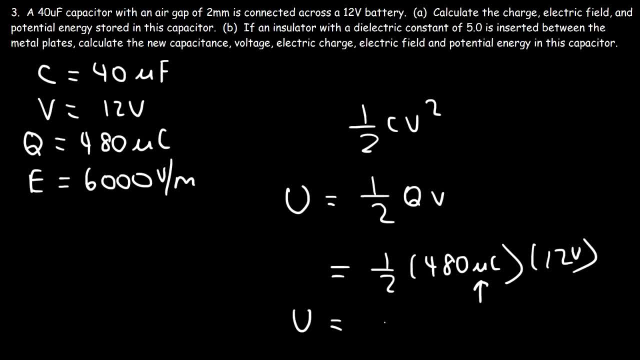 be in a micro. this answer is in millijoules. I mean micro joules. so this is 28, 80 micro joules, which, if you multiply that by a thousand, that's 2.88 millijoules. so that's the potential energy stored in this capacitor. 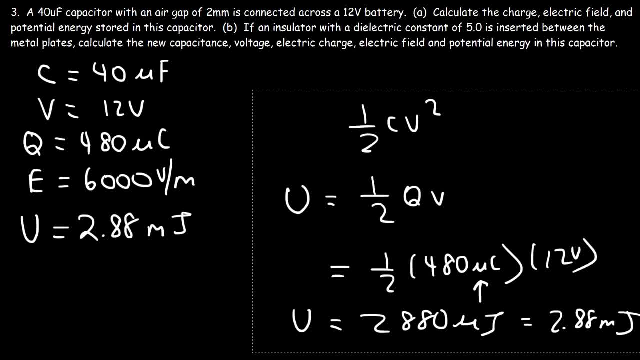 now let's move on to part B. so if we add an insulator with a dielectric constant of 5, what's going to be the new capacitance, voltage, electric charge, electric field and potential energy in this capacitor? well, we know that the capacitance will increase. the new capacitance is going to be the original. 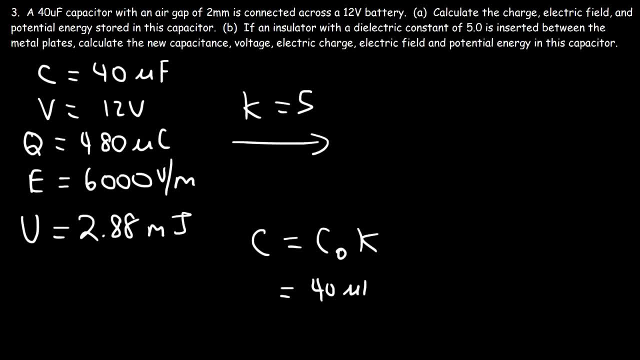 one times K, so it's gonna be 40 microfarads multiplied by 5, so it's gonna increase by a factor of 5, so it's gonna be 200 microfarads. now what about the voltage? because it's still in contact with the battery, the voltage is. 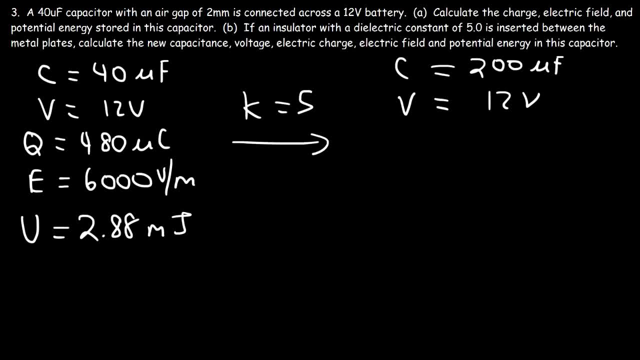 gonna stay the same. initially the voltage drops by a factor 4, so 12. I mean by a factor of 5. 12 divided by 5 is 2.4. but then the battery is going to recharge the capacitor back up to 12 volts, so in the end the voltage will. 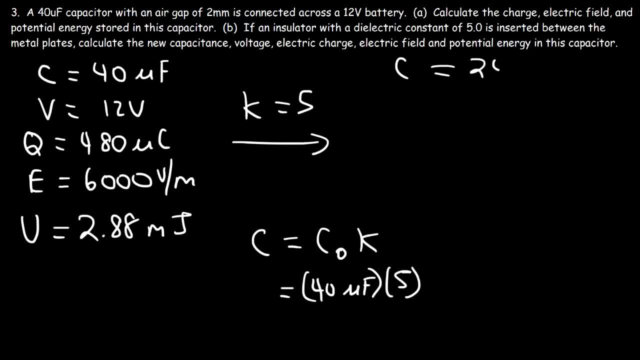 So it's going to increase by a factor of 5.. So it's going to be 200 microfarads. Now what about the voltage? Because it's still in contact with the battery, the voltage is going to stay the same Initially. 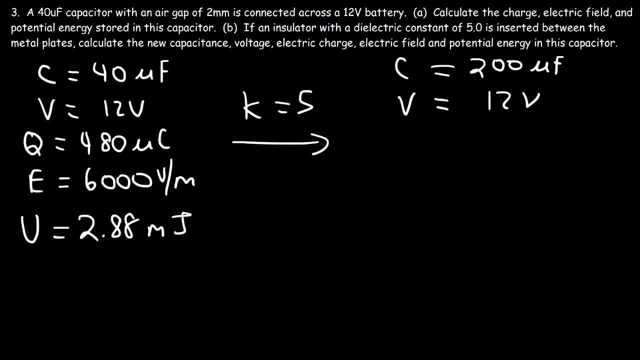 the voltage drops by a factor of 4, so 12. I mean by factor 5. 12 divided by 5 is 2.4, but then the battery is going to recharge the capacitor back up to 12 volts, so in the end the voltage will. 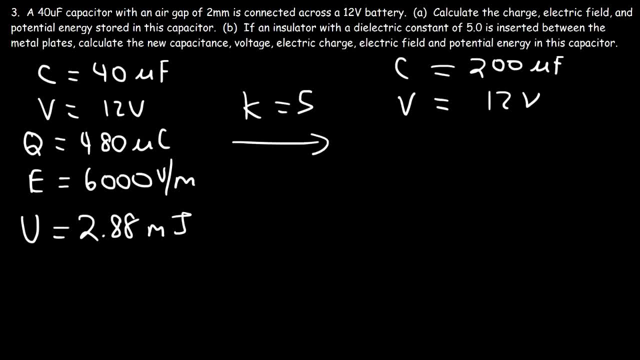 still be 12 because it's still connected to the same battery. now, this time the charge is not going to be constant, it's going to change and the charge is Q equals CV. so see, this time is 200 microfarads and the voltage is 12. so if you take 200 and multiply by 12, that will give you a charge. 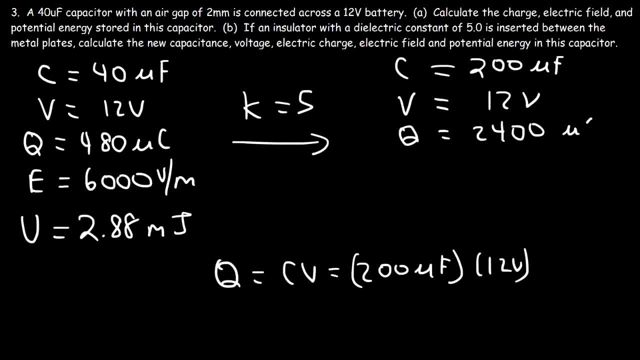 of 2400 microcouple now, because the voltage is still the same, the electric field will be the same. it's going to be 12 volts divided by point zero, zero, two meters, and so it's still going to be 6000 volts per meter. now what about the potential energy? that's 1 half QV, so V is 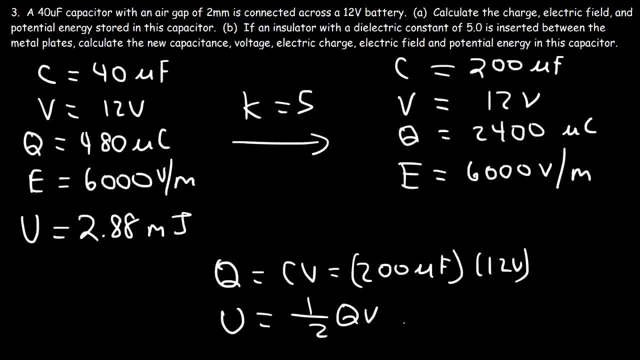 constant, but Q end up, which means the potential energy should go up as well. so it's going to be 1 half times 2400 micro coulombs multiplied by a voltage of 12, and so that's going to be fourteen thousand four hundred micro joules. 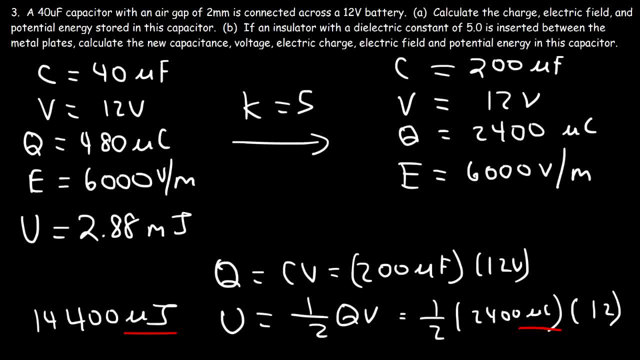 so this is in micro coulombs, this will be in micro joules, and if we divide that by a thousand, this is going to be fourteen point four millijoules, and so that's it. so notice that the capacitance increased by a factor of five and a potential energy increased by a factor five. it's two point. 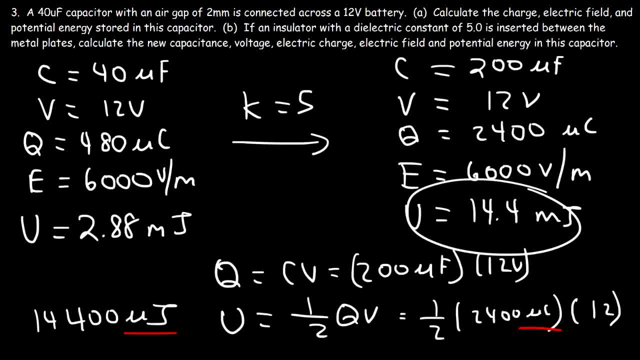 eight, eight times five. so the increase in potential energy came from the battery. once you add the insulator, the voltage of the capacitor goes down, and so there's going to be a difference between the voltage of the battery and the voltage of the capacitor, and so the 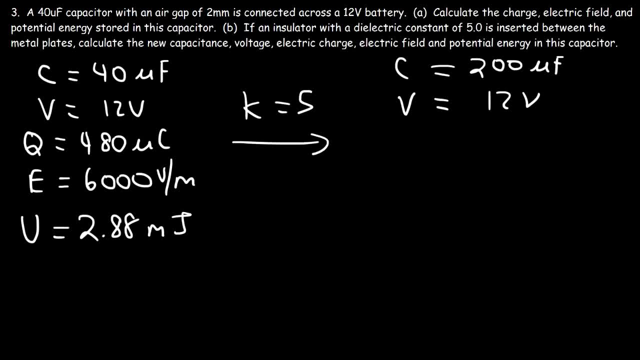 still be 12 because it's still connected to the same battery. now, this time the charge is not going to be constant, it's going to change and the charges Q equals CV. so see, this time is 200 microfarads and the voltage is is 12.. So if you take 200 and multiply it by 12, that will give you a charge of 2400. 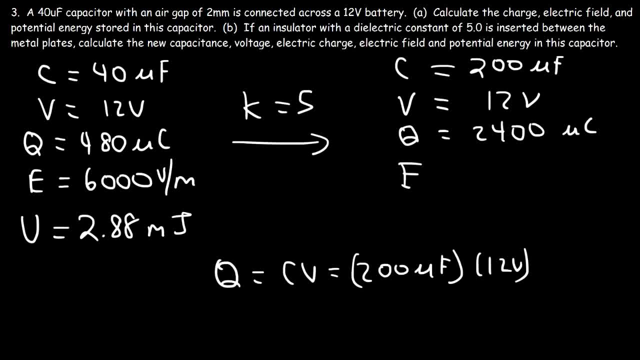 microcoulombs. Now, because the voltage is still the same, the electric field will be the same. It's going to be 12 volts divided by 0.002 meters, and so it's still going to be 6000 volts per meter. Now what about the potential energy? That's 1 half QV, So V is 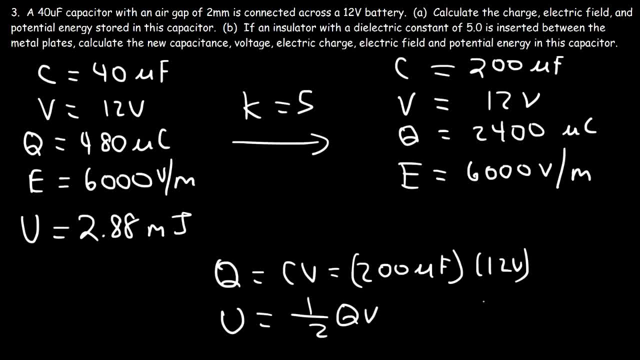 constant, but Q end up, which means the potential energy should go up as well. So it's going to be 1 half times 2400 microcoulombs, multiplied by a voltage of 12. And so that's going to be 14,400 microjoules. So if this is in microcoulombs, this will be in microjoules, And if we divide, 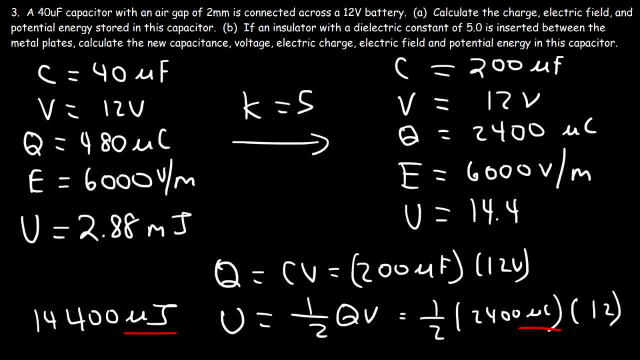 that by 1000, this is going to be 14.4 milliamps, And so that's it. So notice that the capacitance increased by a factor of 5, and the potential energy increased by a factor of 5.. It's 2.88 times 5.. So the increase in potential energy. 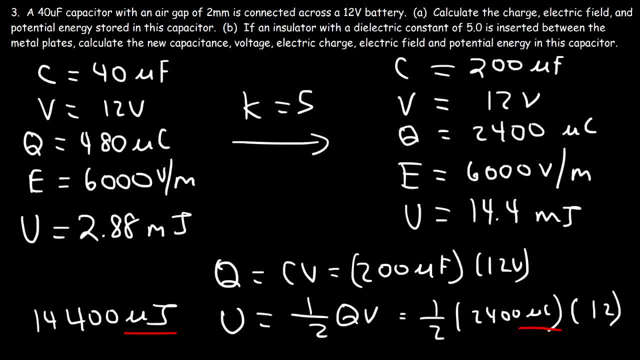 came from the battery. Once you add the insulator, the voltage of the capacitor goes down, And so there's going to be a difference between the voltage and the voltage of the capacitor, And so the battery charges up the capacitor back to 12 volts, And that's why the potential 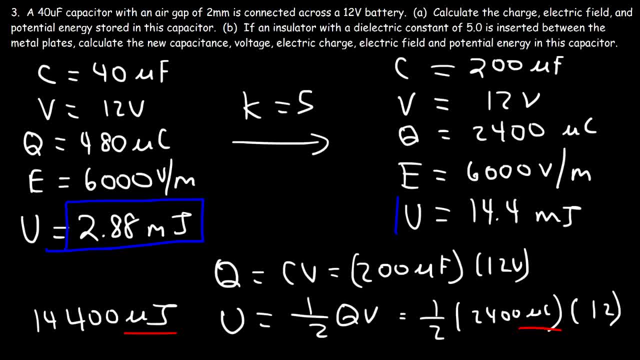 energy goes up because more energy is consumed from the battery once you add the insulator. So let's summarize everything for this problem. So if the capacitor remains in contact with the battery, if we increase the dielectric constant, the capacitance will increase.